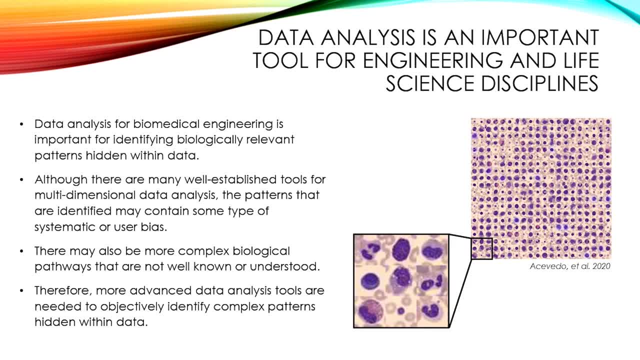 Data analysis is an important tool for engineering and life sciences. Data analysis for biomedical engineering is important for identifying biologically relevant patterns that might be hidden within the data. There are many established tools for multidimensional analysis, but the patterns that those identify might contain some kind of bias and there may be more complex biological pathways that are not well known or understood. 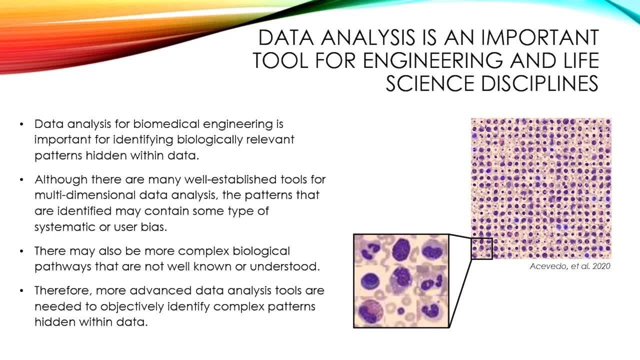 Therefore, we want to use some more advanced data analysis tools to objectively identify complex patterns that could be hidden within the data. This figure contains images of different cell types that require years of training to identify, and even then the identification is still prone to human error. 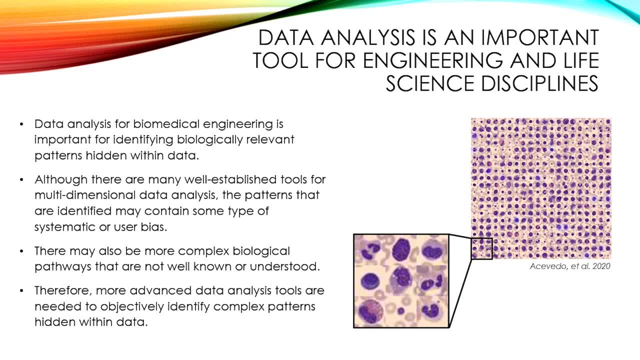 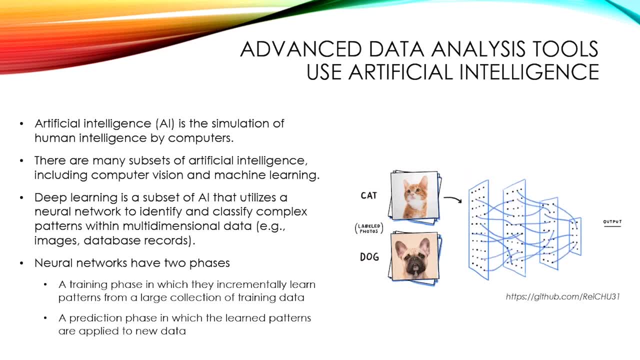 This identification could be handled by a computer in a more objective way. Advanced data analysis tools use artificial intelligence. Artificial Intelligence, or AI, is the simulation of human intelligence by computers. There are many subsets of AI, including computer vision and machine learning. 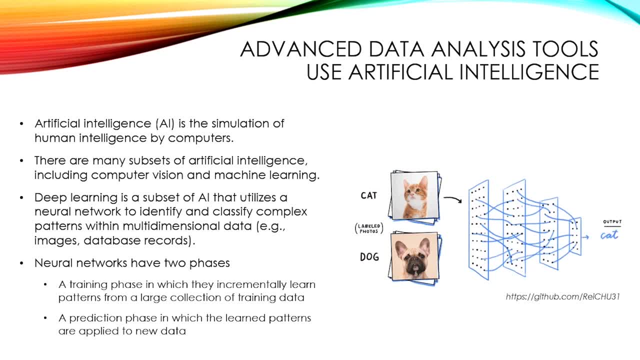 Deep learning is a subset of AI that utilizes a neural network to identify and classify complex patterns within multidimensional data, for example, images or database records. Neural networks have digital data and graphical analysis to exclude These data items when used for photographic and visual study and on a multidimensional scale. 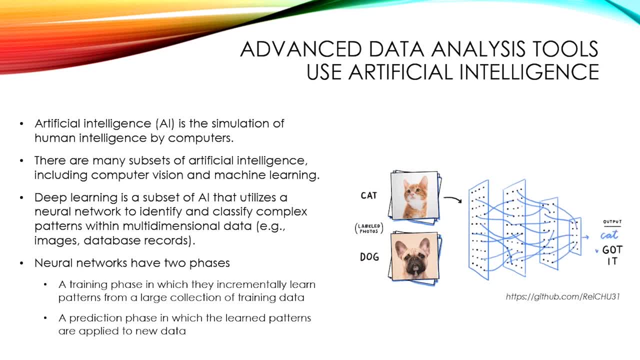 Neural networks have digital data and graphical analysis tools, to called neural networks, which are composed of complex Western Hills data from which that network acts, Neural networksаноid networks ecosystem and Porqueh Mittel primera informender professional data system. two phases: a training phase in which they incrementally learn patterns from a large 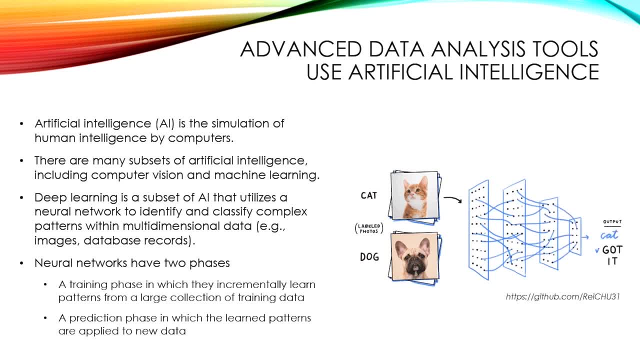 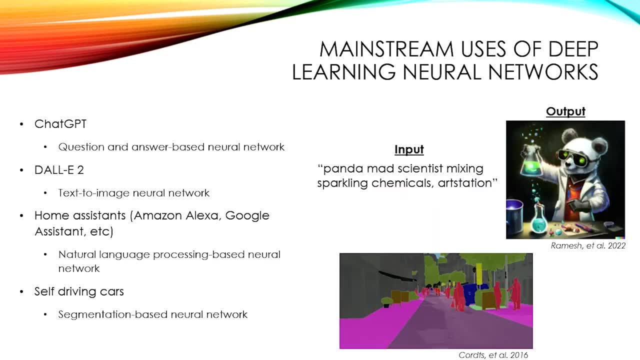 collection of training data and a prediction phase in which the learned patterns are applied to new data. There are many mainstream uses of deep learning neural networks. ChatGPT is a question and answer based neural network. DOL-E2 is a text-to-image neural network and on the right you can see a sample input. 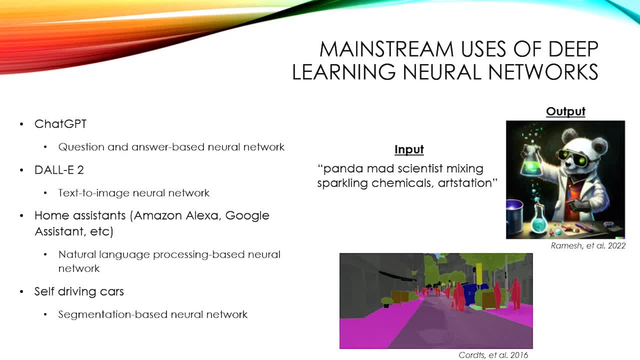 and the sample output of this system And also our home assistants, Amazon Alexa, Google Assistant, et cetera- are natural language processing-based neural networks And also, of course, self-driving cars, where they use computer vision and route planning. 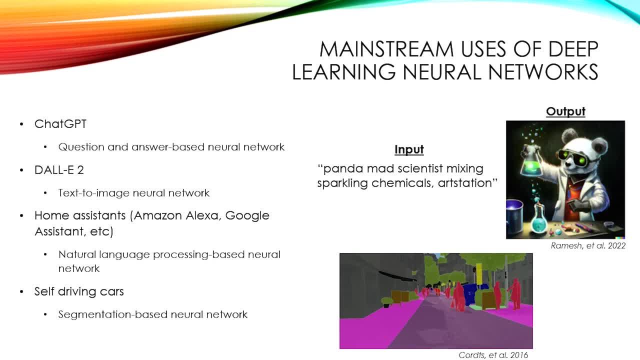 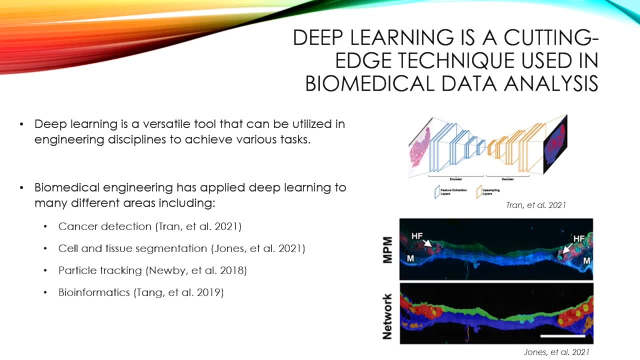 to navigate through the scene and to the right, you can see a picture of what those neural networks process. Deep learning is a cutting-edge technique used in biomedical data analysis. It's a versatile tool and biomedical engineering has applied deep learning to many different. 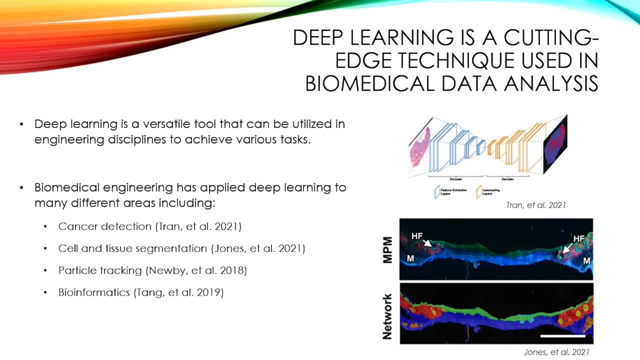 areas including cancer detection, cell and tissue segmentation, particle tracking and bioinformatics. To the right, we see an image of a network architecture that can be used to detect cancer sites in thin sections of tissue. Beneath that there's a pair of images: an input image and an annotated bottom image. 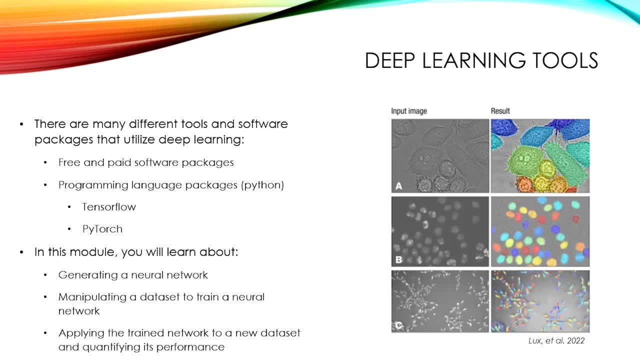 of a wound site in a thin tissue section. This is an image of a wound site in a thin tissue section. There are many deep learning tools. These might be in the form of free and paid software packages or just add-ons to existing programming languages like Python, such as TensorFlow and PyTorch. 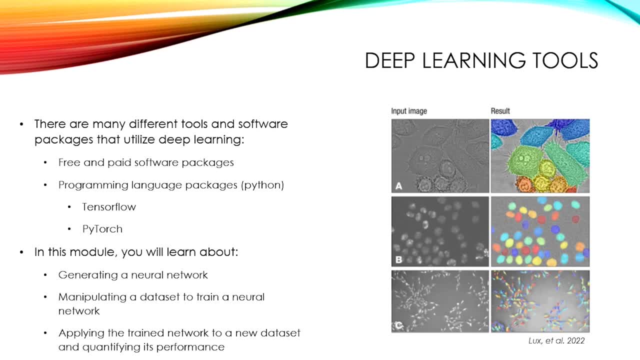 In this module, you'll learn about generating a neural network, manipulating a data set to train a neural network, applying the trained network to a new data set and quantifying its performance. The figure contains input images on the left And corresponding segmented images on the right. 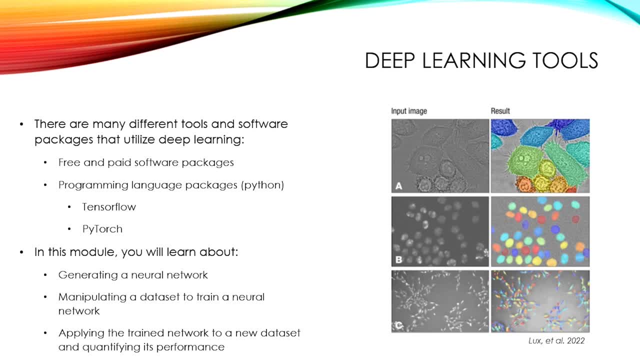 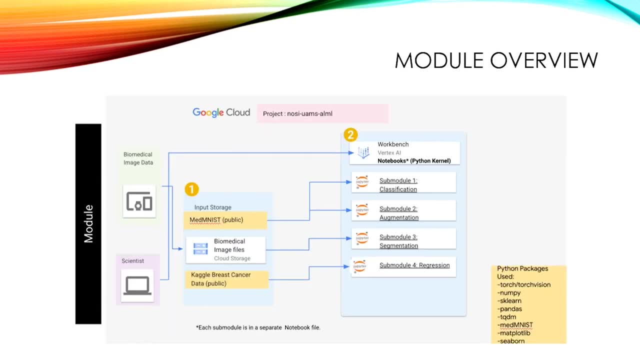 This network was trained using an add-on to ImageJ, a free image analysis program from the NIH. This diagram provides an overview of the module's organizational structure. You will use biomedical image data stored in the cloud, as well as two public data sets. 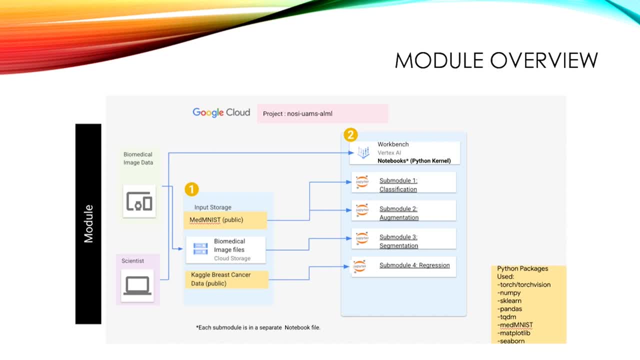 MED-EM, NIST and the Kaggle breast cancer data. You will interact with a Vertex AI workbench And during the module you will use a variety of Python packages, including Torch, TorchVision, NumPy, sklearn, pandas and several others. 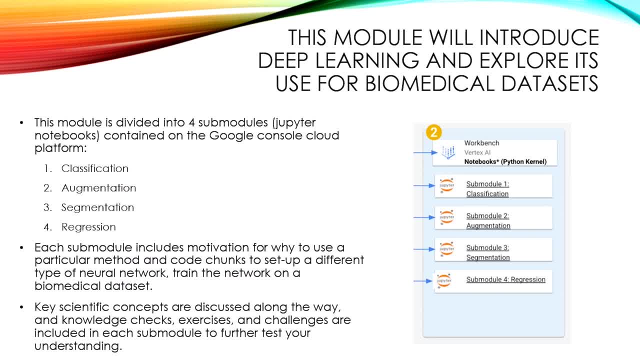 This module will introduce you to deep learning and explore its use for biomedical data sets. The module is divided into four sub-modules, each in a Jupyter notebook, which are contained on the Google console cloud platform. The sub-modules are Classification, Augmentation, Segmentation and Regression. 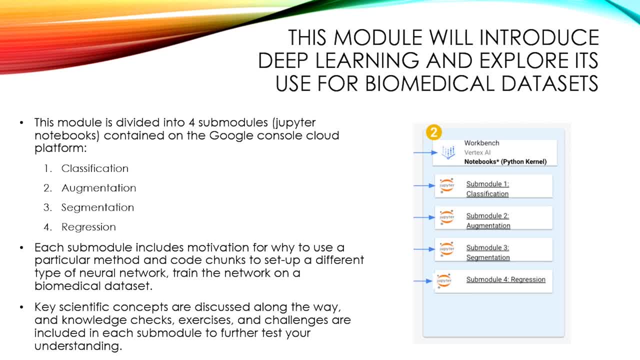 Each sub-module includes motivation for why to use that particular method and code chunks to set up a different type of neural network, train that network on a biological data set. Key scientific concepts are discussed along the way and there are knowledge checks exercises. 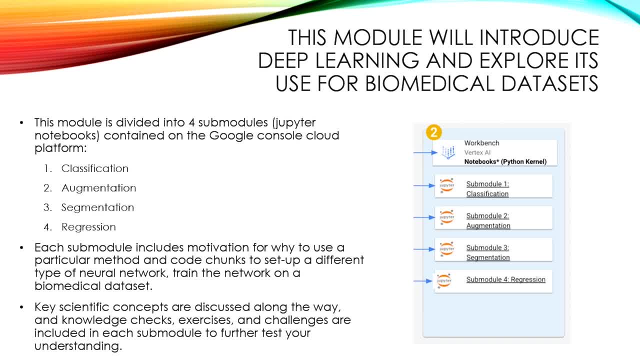 and challenges in each sub-module to further test your understanding. So how can you get the most out of the MED-EM NIST? Well, there are a number of ways to get the most out of the MED-EM NIST. One of the most important ways to get the most out of the MED-EM NIST is to get the most. 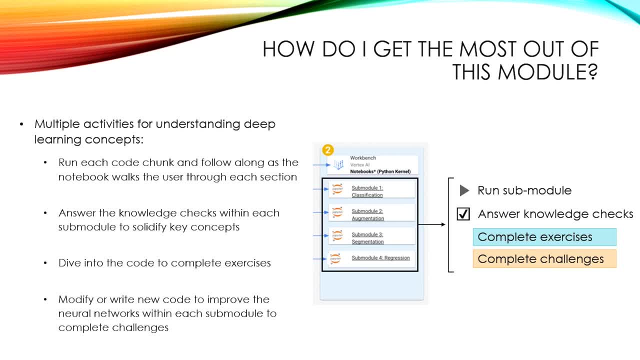 out of this module. There are multiple activities available for understanding deep learning concepts. Each sub-module has code chunks that you can run and you can follow along as it walks the user through each section. You can answer the knowledge checks within each sub-module to identify the key concepts. 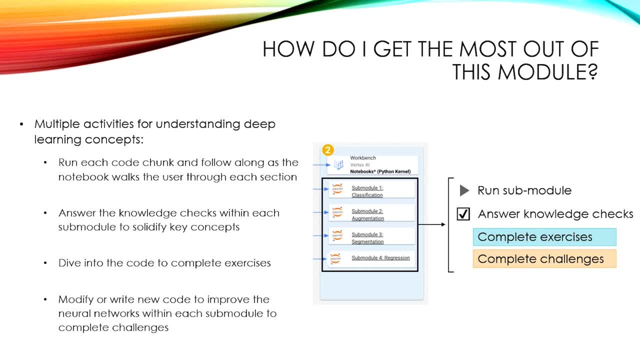 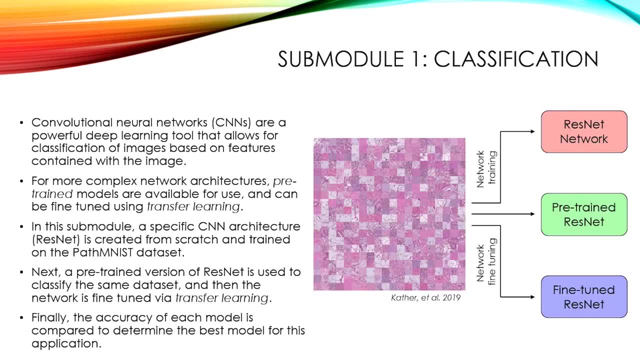 You can dive into the code and complete exercises and you can modify and write new code to improve the neural networks within each sub-module to complete challenges. The first sub-module is Classification. Convolutional neural networks are a powerful deep learning tool that allows for. 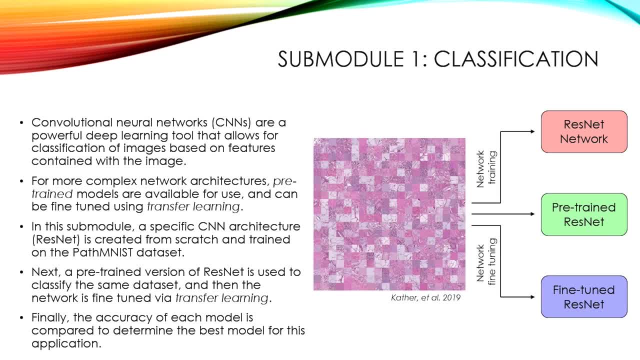 classification of images based on features contained within the image. For more complex network architectures, pre-trained models are available and they can be fine-tuned using transfer learning. In this sub-module, a specific CNN architecture called ResNet is created from scratch, and 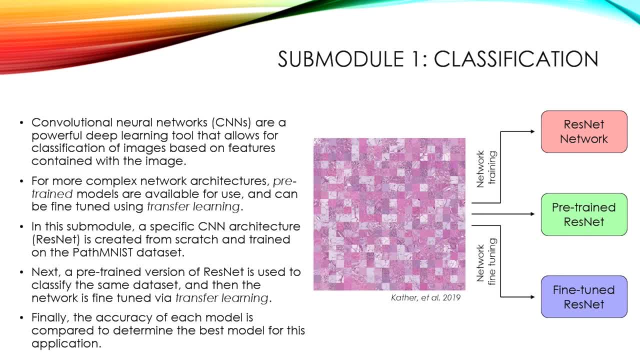 trained on the PATH-M NIST dataset. PATH-M NIST contains pathological images, or images of thin sections of colorectal cancer. In addition, a pre-trained version of ResNet is also used to classify the same dataset, and then the network is fine-tuned via transfer learning. 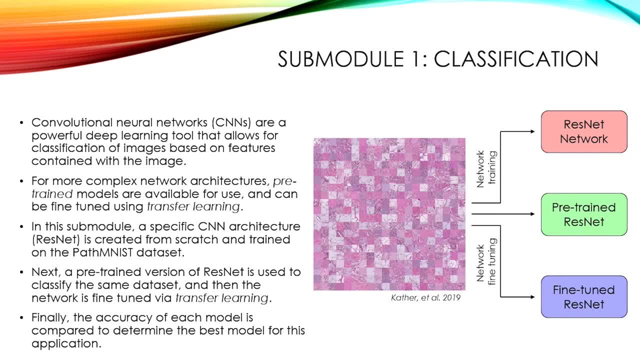 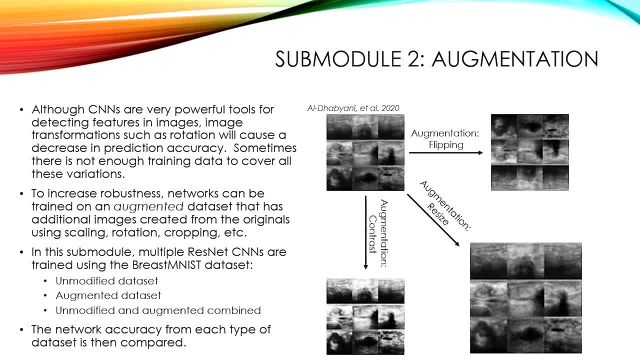 And, finally, the accuracy of each model is compared to determine the best model for this application. Although CNNs are very powerful tools for detecting features in images, image transformations such as rotation will cause a decrease in prediction accuracy. Sometimes there is not enough training data to cover all these variations. 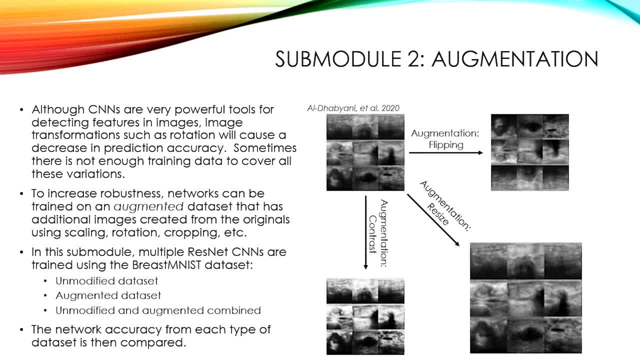 To increase robustness, networks can be trained on augmented data sets that have additional images created in them from the originals, using scaling, rotation, cropping, etc. In this submodule, multiple resonant CNNs are trained using the Brest MNIST dataset.